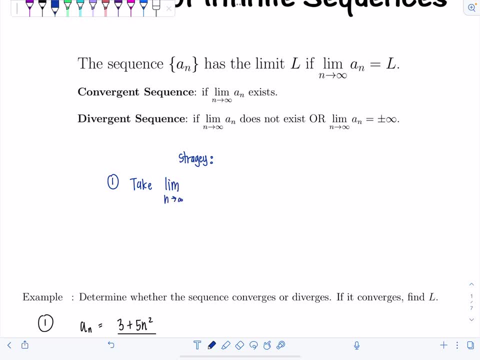 directly. So you take the limit as n approaches infinity of a n directly and you hope that you get a number or infinity. negative infinity does not exist and you're done. If that doesn't work, okay, some other things you can do. You can define a function that is basically equivalent to your sequence and then you're going to use 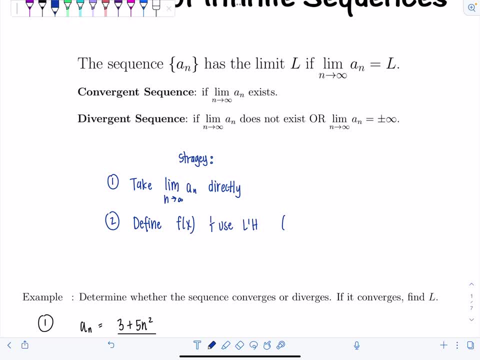 L'Hopital's rule, if you have the case of zero over zero or infinity over infinity, etc. Another option is you can apply the squeeze theorem or sandwich theorem. Usually that'll come up when you're doing a series of equations. So you can do a series of equations and you can. 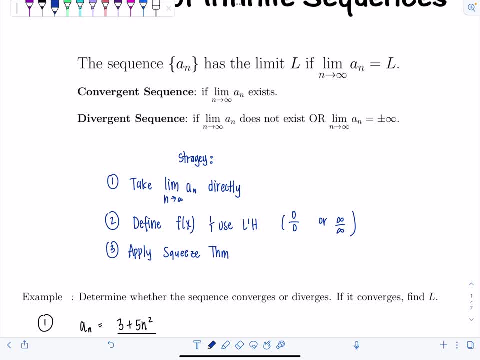 move up the character, because you could avoid that. You can also do a series of equations, and then you can do a series of equations. that will be similar to how you can do a sequence, and then you have sequences that involve sines and cosines, because they're easily bounded. 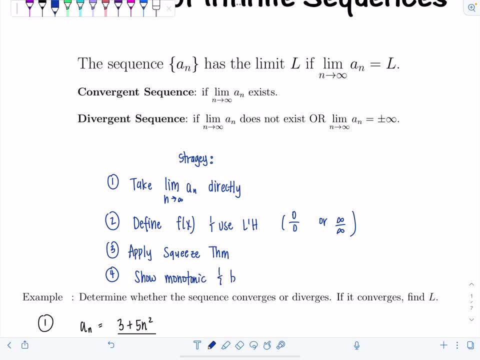 And the last thing you can try to do to show a sequence is convergent is to show that it's monotonic and bounded. Now there's a whole other discussion that needs to be had about that, so I'll link a video here where I do it precisely said discussion. Okay, so let's just jump into some examples. We'll warm up with some easy ones here and we'll show you some examples of what a sequence looks like for a sequence. 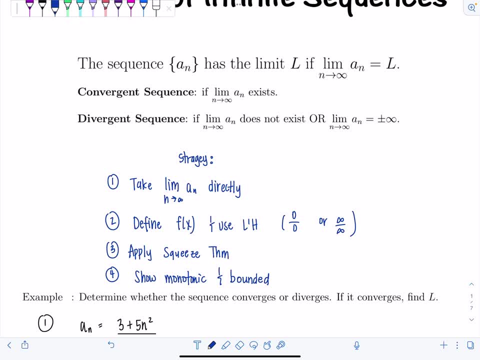 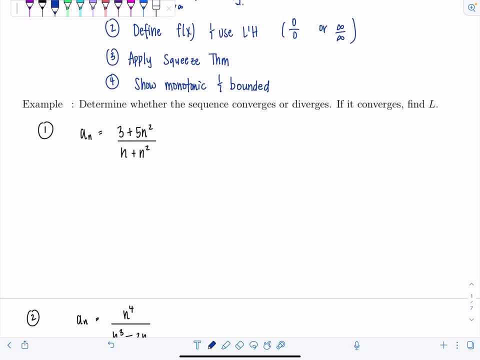 Okay. so let's just jump into some examples. We'll warm up with some easy ones and then we'll kick up the spice level at the end. So here we go: Determine whether the sequence converges or diverges. If it converges, find L. So I'm just going to start off. take the limit. 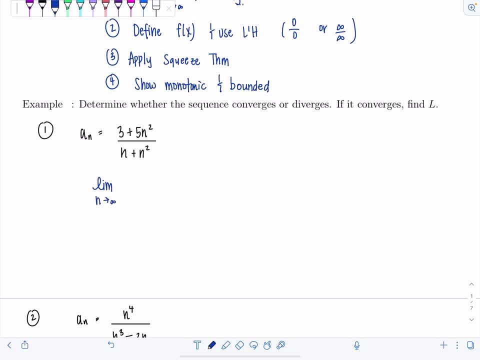 as N approaches infinity, and see what emerges. If this doesn't work out for me, then I'm going to go through my strategy list, okay, So here we have a rational expression, rational function Divide by the highest power of N that you see in the denominator. So in this: 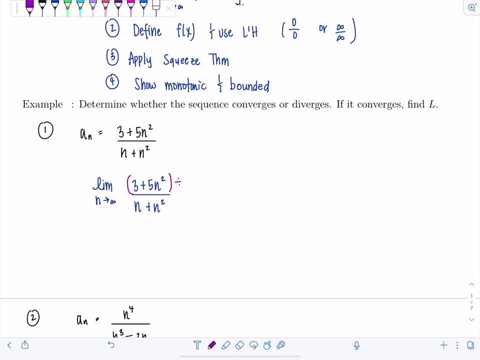 case that would be N squared. So I'm going to divide everybody by N squared And then in the next step let's see what we got. So we've got limit. N approaches infinity, Infinity. In the numerator I'm going to have 3 over N squared plus 5.. 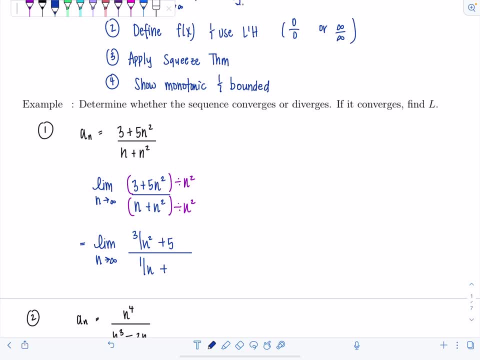 N over N squared, that's just 1 over N, and then plus 1.. All right, so as N approaches infinity, 3 over N- squared, that's going to go to 0.. 5 is just a constant, And then 1 over N also approaches 0.. So all we're left with is 5 over 1,. 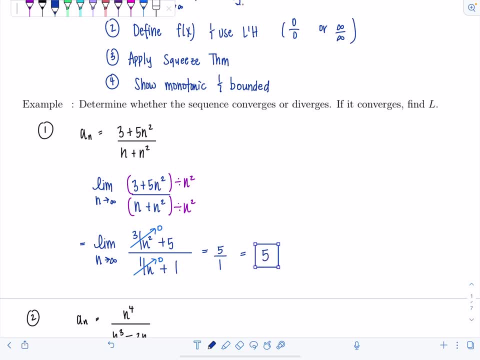 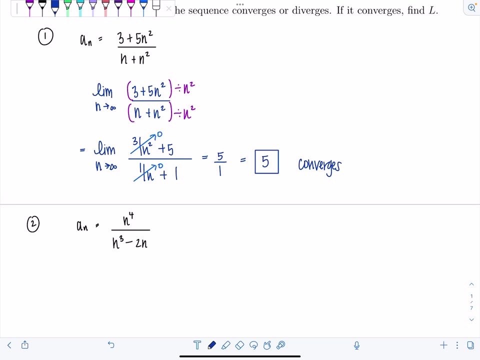 which is 5.. So that's my limit. L, That's a finite number. So that tells me that this sequence converges And that's it. Okay, Let's look at another one. See, they're not so bad. The sequence AN is N to the fourth over N, cubed minus 2N. So we're going to take the limit. 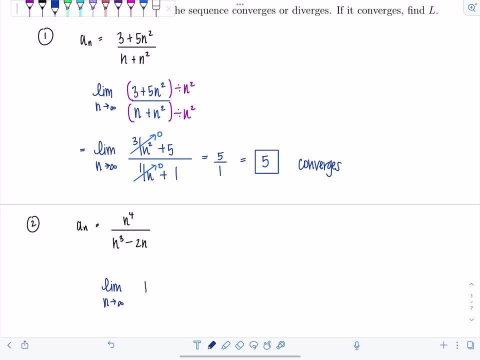 as N approaches infinity. This is always my first go-to. Just take the limit of the term. see what's happening? So we're going to take the limit. as N approaches infinity, So we're going to take the limit of the term. 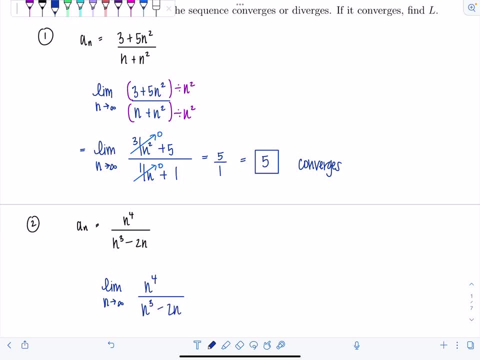 N to the fourth over. N squared minus 2N, N cubed minus 2N. Now be careful: You only divide by the highest power of N from the denominator, Not overall. No, no, no. So highest power of N from. 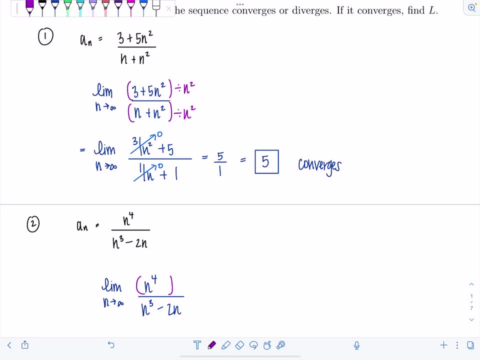 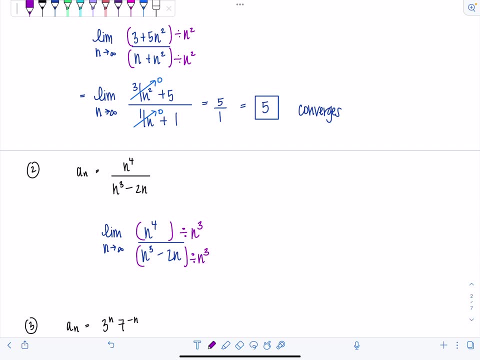 the denominator again is N cubed. So let's go ahead: divide by N cubed. And now we've got, let's see, limit N approaches infinity N to the fourth, divided by N cubed. N cubed divided by N cubed is just N N cubed divided by N cubed is 1 minus. I'm going to have 2 over N squared. 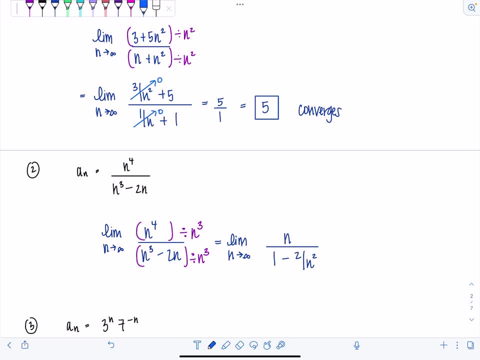 So now let's see what's going on As N approaches infinity. the numerator has an N, So that's going to go to infinity. Denominator 1 is just a constant minus 2 over N squared, That's going to go to 0.. 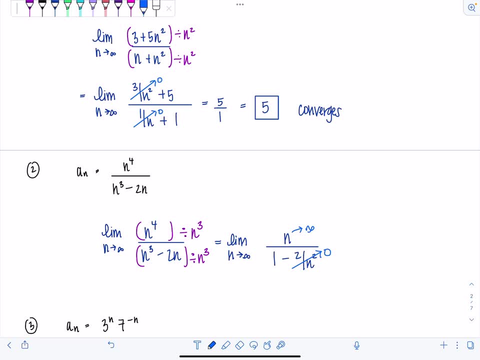 So now I have numerator approaches infinity, infinity denominator approaching one, a positive constant. so this limits going to be positive infinity. well, that's a limit, but it's not L, because L is only defined to be a finite number. okay, so this sequence diverges and we leave it. 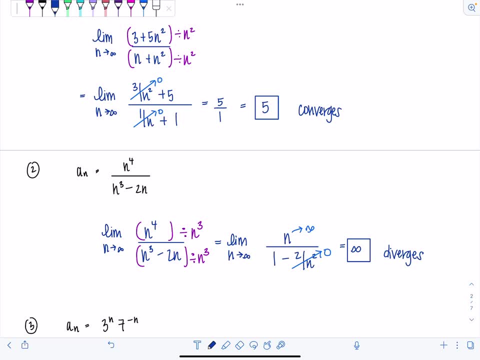 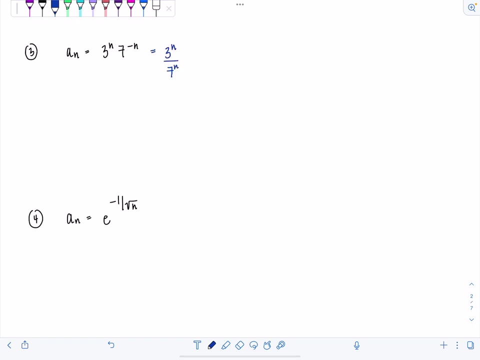 alone. okay, look see, we're surviving, we're thriving. let's move on to example three. a n equals 3 to the n times 7 to the negative n. I'm gonna rewrite this, sucker, okay, before I take the limit. this is 3 to the n over 7 to the n which I 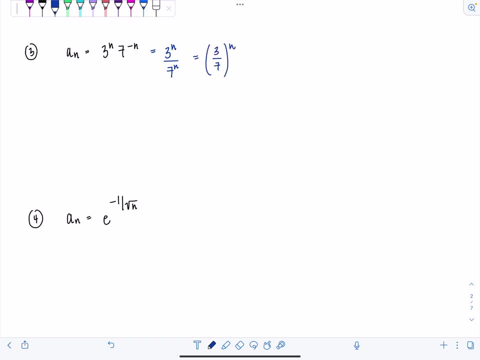 can rewrite as 3 sevenths to the n. okay, now let's take the limit, as n approaches infinity, of 3 sevenths to the n. this limit, hopefully you're familiar with it. this is a geometric sequence and the common ratio R is equal to 3 sevenths, which is less than 1. so this: 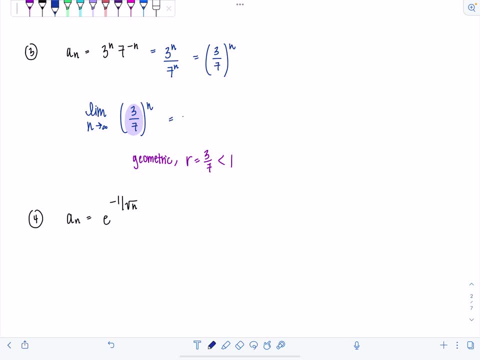 limit is going to be 0, why? let's think about it. you're taking 3 sevenths, something smaller than 1, and you're multiplying it by itself infinitely many times. it's going to keep shrinking, shrinking, shrinking, shrinking, approaching 0, and that's the case for any geometric 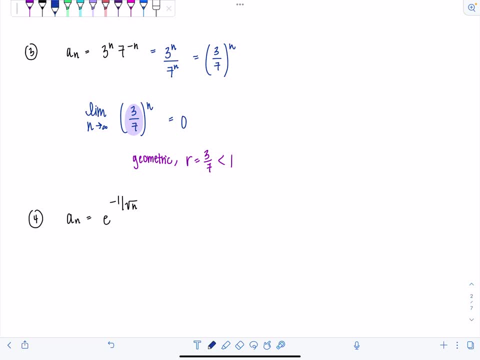 sequence when R is less than 1. so that's our limit, L, and we can say that this sequence converges. that's it, okay, okay, okay. example for a: n equals e raised to the negative 1 over rad M. so here we go, let's take the limit. 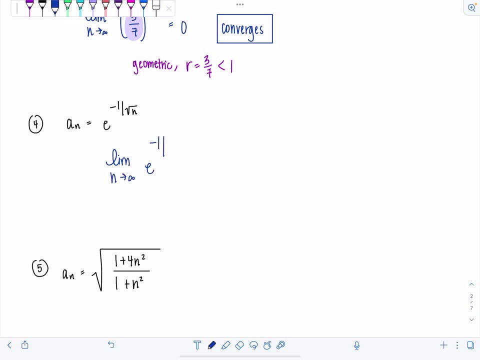 as n approaches infinity, of e to the negative 1 over rad M. e raised to the x is a continuous function, so I'm gonna apply one of my limit laws for sequences and pass the limit through to the exponent. so watch how I'm going to rewrite it. it's so slick. you have e raised to the limit as n approaches infinity and n approaches infinity, so we can do this again. 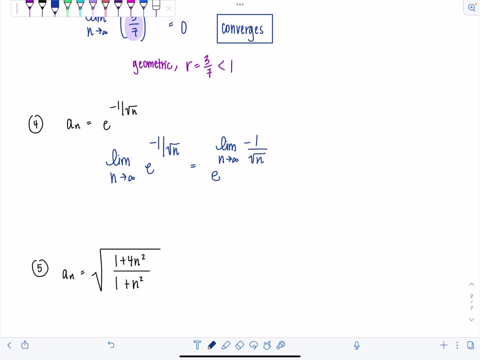 of negative 1 over rad n. Okay, so let's see what's going on here. As n approaches, infinity denominator is getting really, really big. So negative 1 over rad n, that's going to approach 0.. So now for my limit. I'm left with e to the 0, which is 1.. Well, that's a finite number. That's l. 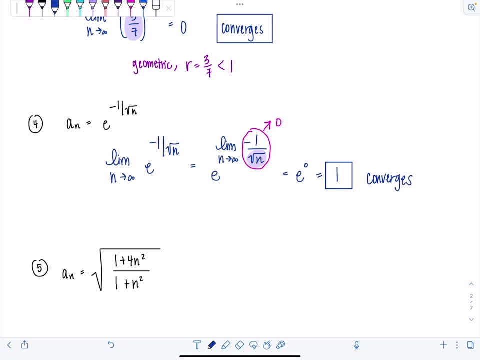 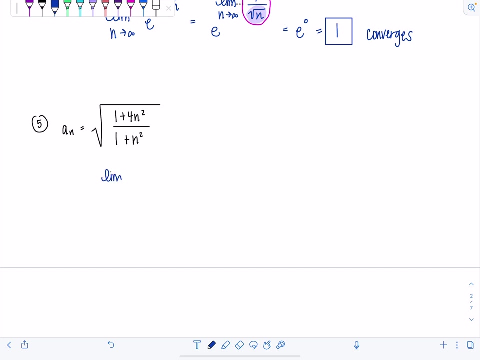 So this sequence converges. Okay, good, Let's look at another Example: 5.. a? n equals square root of 1 plus 4 n squared over 1 plus n squared Every single time. start off limit. n approaches infinity: Square root 1 plus 4 n squared. 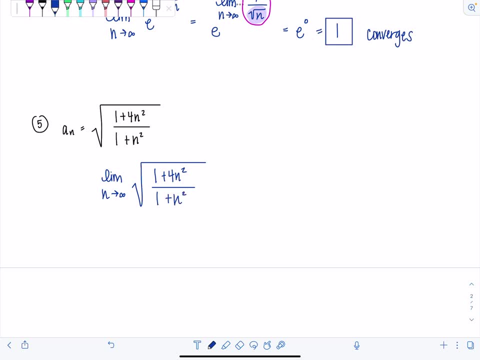 over 1 plus n squared. So this sequence converges. So, similar to the last example that we did, we're gonna apply our limit laws and I can pass the limit underneath the radical, Since n is approaching infinity, positive, infinity right. 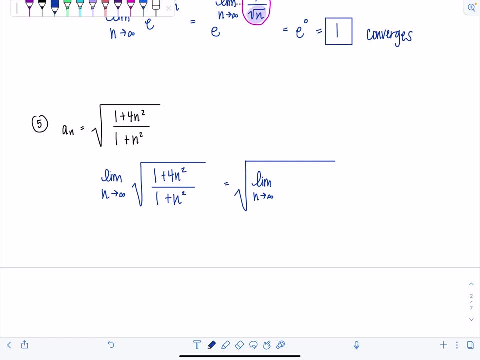 Always with these sequences. I know that the radical is going to be well-defined. I'm not gonna have any negative values underneath, so I can pass that limit underneath. And now let's see, we've got one plus four n squared over one plus n squared. 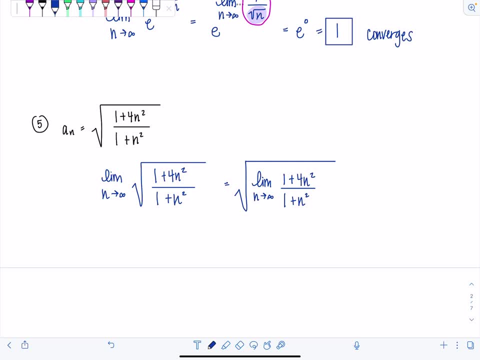 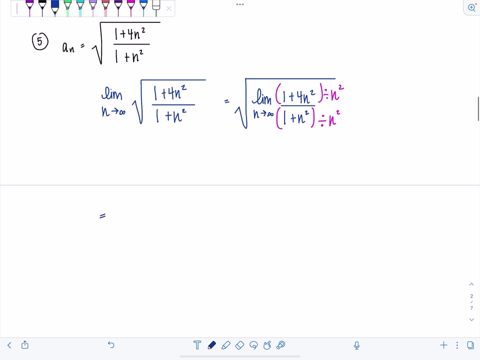 plus everything squared under the radical. so we're super duper safe. Now I'm just gonna focus on this rational expression. Let's divide numerator and denominator, this time by n squared, That's the highest power of n in the denominator. And then we've got here square root of the limit. 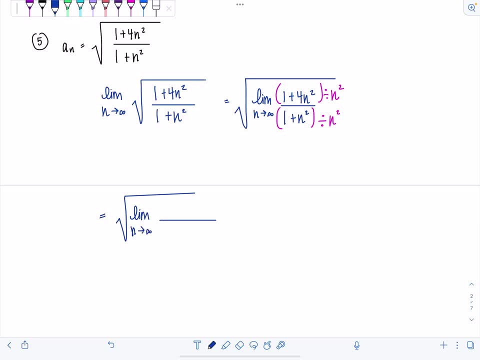 as n approaches infinity, we will have one over n? squared, plus four over one over n squared, plus one Beautiful. So as n approaches infinity, these one over n squareds go to zero, And I'm just left with four over one. underneath the radical. 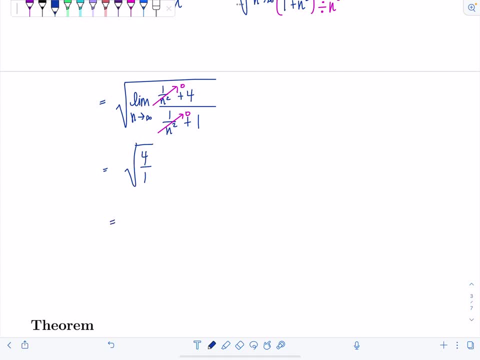 but that's just square root of four right, Which is two, So that's a finite number, so that's l, And we can say that this sequence converges. Okay, Now, before we move on to the next couple examples. 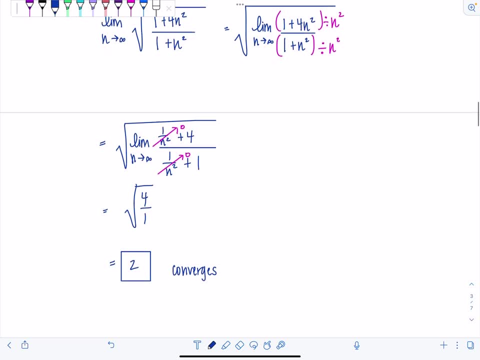 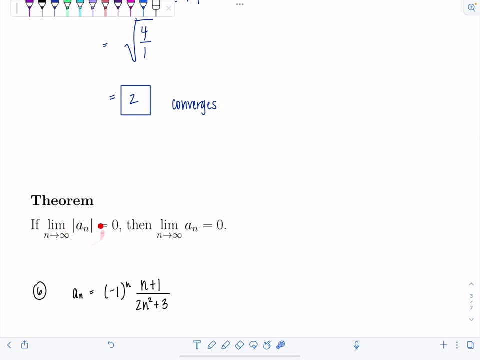 I wanted to show you or remind you of a theorem. It states: if the limit of n approaches infinity of the absolute value of a, n is equal to zero. then the limit of n approaches infinity of original original an without absolute value is also equal to zero. And I explained this more a little bit. 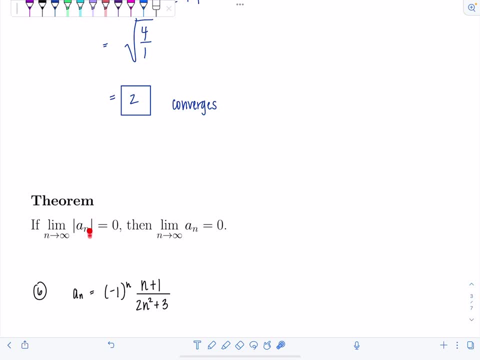 in the lecture why that's the case. But basically, if you take the absolute value of the terms and they approach zero, that means they're shrinking in magnitude. right, Absolute value makes everything positive if it isn't already, or zero, worst case scenario. So if the limit of 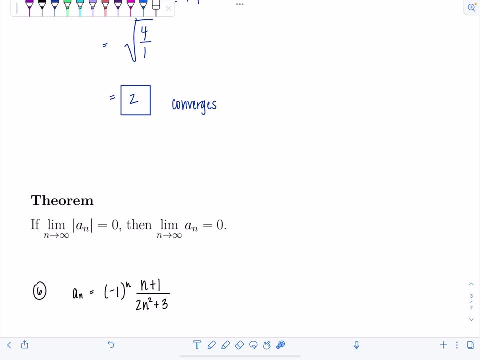 everything when it's not negative shrinks to zero. then, even if the terms bounce between being positive and negative, they are shrinking in magnitude and will approach zero as well. Why am I reminding you of this? This is great to use anytime you have an alternating sequence. 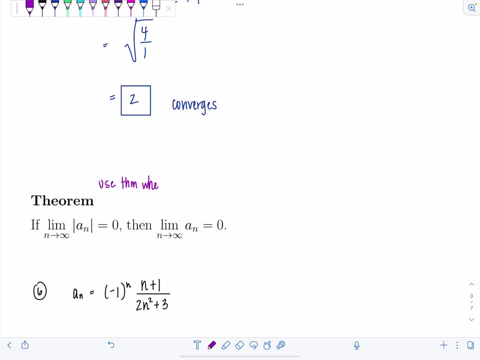 So use this theorem when an involves negative one to the n or negative one to the n plus one, and then it has some other stuff, okay, Like the following example right here: So an equals negative one to the n Times n plus one over two, n squared plus three. So how would you write this up properly? I will 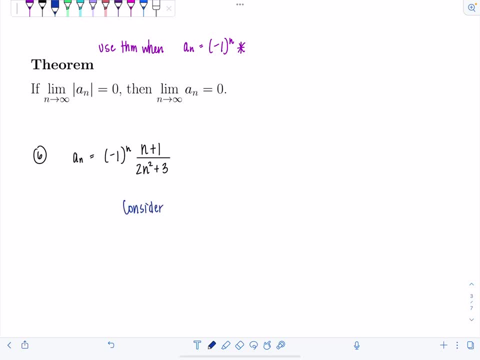 show you. You should say: consider the absolute value of an, which is equal to the absolute value of negative one, to the n of n plus one over two, n squared plus three. Well, what is taking the absolute value do? It basically eliminates this alternating portion, because now negative one to. 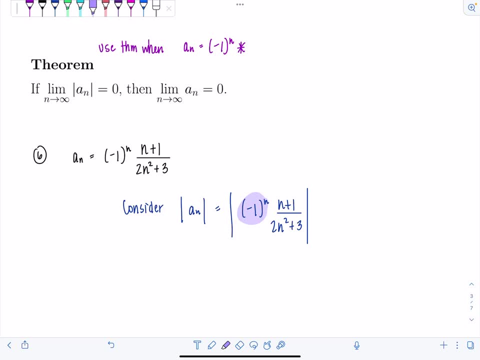 n is equal to the absolute value of n plus one over two, n squared plus three. So now let's go ahead. I'm going to take the limit not of the original sequence, but of the absolute value of an, And let's see what happens. I'm feeling optimistic. 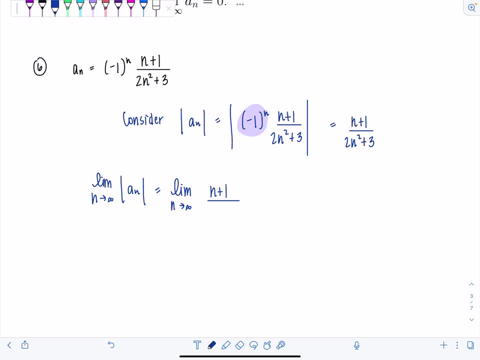 Limit, as n approaches infinity, of n plus one over two, n squared plus three. Now how do we take this limit? Don't even say L'Hopital's rule, because then we have to define a function and it's so much more work. So we're going to divide by the highest power of n in the denominator. Divide by: 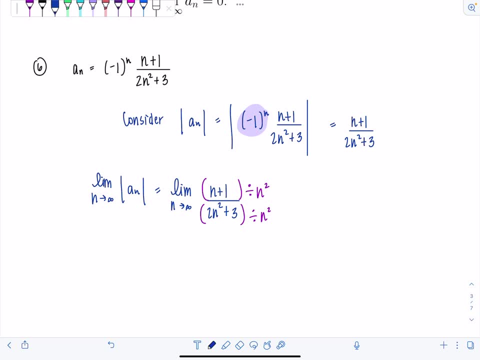 n squared. And then let's see, We've got the limit as n approaches infinity: n over n squared, though, That's one over n plus one over n squared. And then down here we have two plus three over n squared. Okay, One over n is going to zero. One over n squared also goes to zero, Same as three over n. 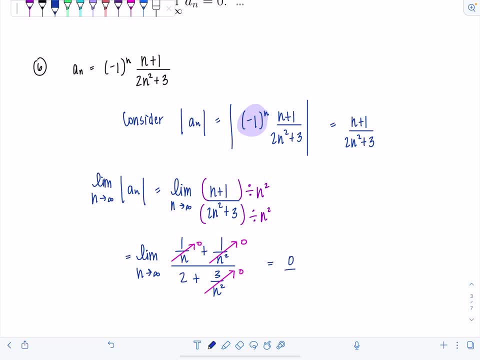 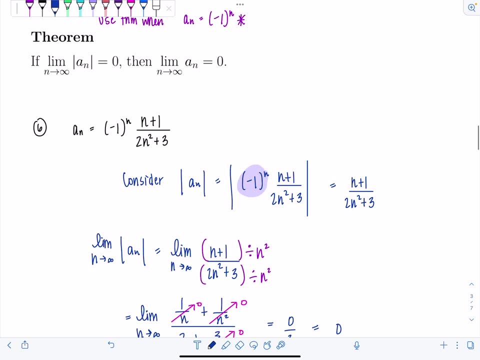 squared. So all I'm left with now is zero over two, which is zero. I'm so excited because remember what did my theorem say: If the limit as n approaches infinity of the absolute value of the terms is zero, then the original limit. 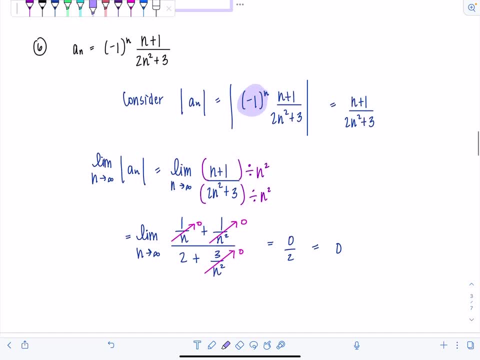 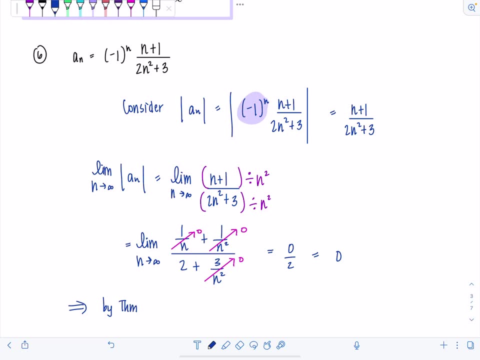 as n approaches infinity of the sequence is also zero. So now I can answer the question. So I can say this implies by said theorem that the limit as n approaches infinity of the original negative one to the n times n plus one over 2 n squared, plus three over n, one over two n squared, plus three over n squared. 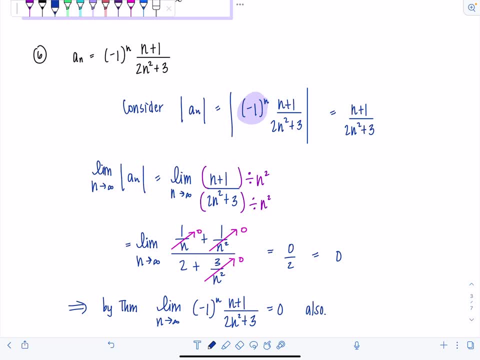 plus three equals zero, also Convergent. Now why did I freak out at you right now about L'Hopital's rule? Because L'Hopital's rule can only be applied to differentiable functions Sequences. I'm so. 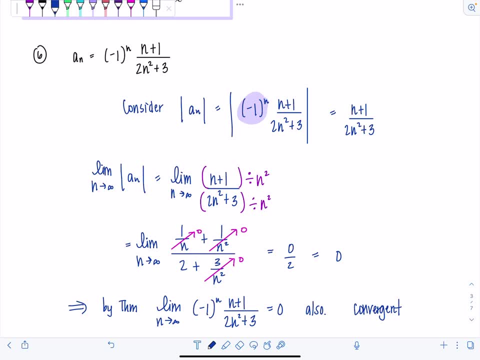 sorry, they're not differentiable right. These are points, a discrete set of points that are not continuous. So you can't apply L'Hopital's rule unless you define a function basically equivalent to the terms of the sequence, and it's just a little bit more work. So I tried to save L'Hopital's. 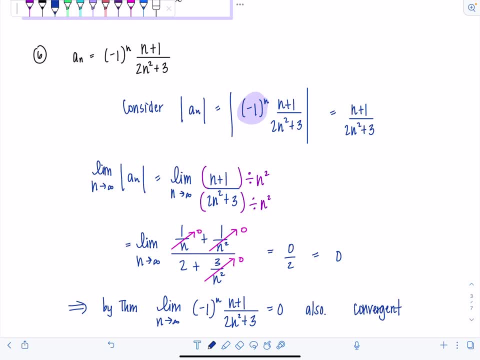 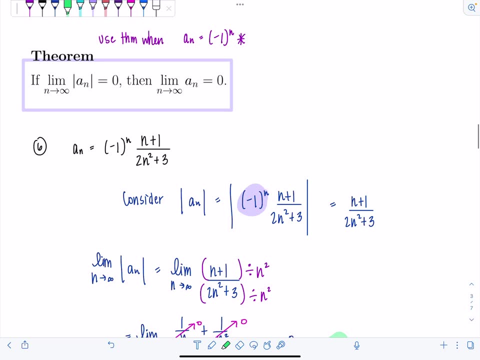 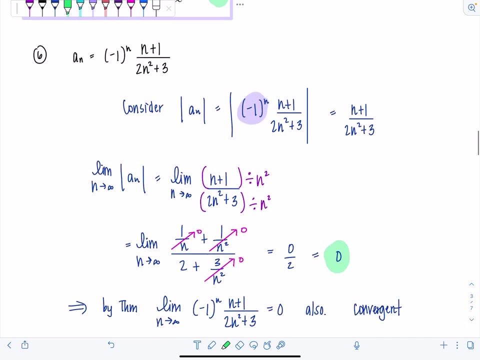 rule for only when it's very, very necessary. okay, Now, this worked out conveniently for us because this limit was zero. yes, What if it is not? What does that tell you? I will show you. It actually means the sequence diverges, But how do you write it up? nicely? Observe the following: 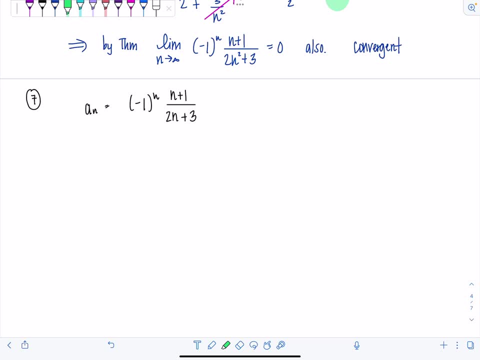 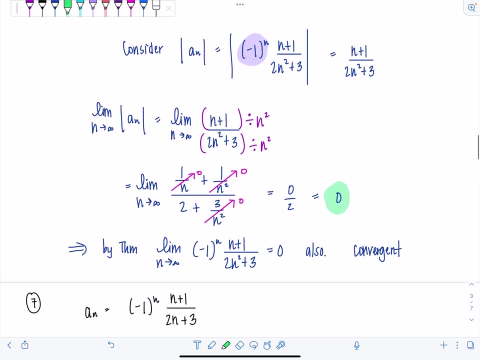 So here's L'Hopital's rule for only when it's very, very necessary. Now, this worked out conveniently for us. So here's something very similar, a sequence I made up. We have a: n equals negative 1 to the n times n plus 1 over 2n plus 3.. See what's the only difference between this example. 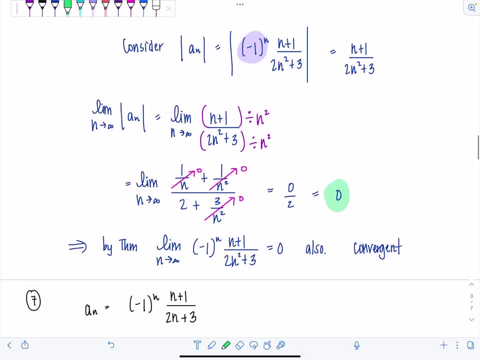 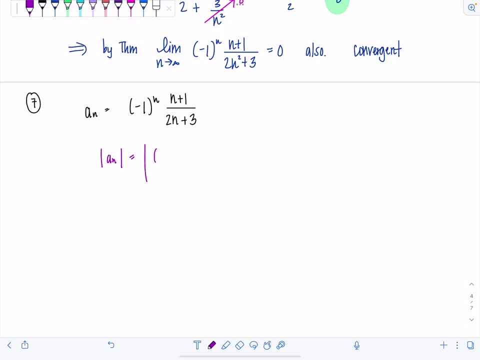 and the one before The n is not squared in the denominator. Oh my, that's going to change everything. So, absolute value of a n, absolute value of negative 1 to the n times n plus 1 over 2n plus 3.. All that happens. 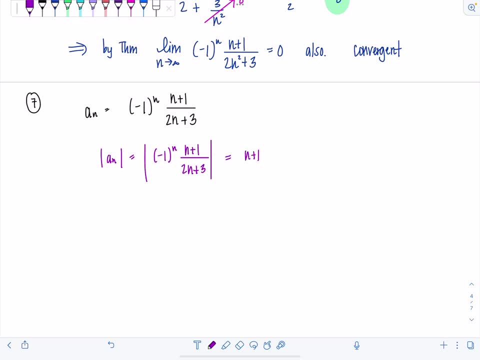 What happens is that alternating portion's gone, So now we just have n plus 1 over 2n plus 3, all right. So now we're going to say: let's consider the limit as n approaches infinity of the absolute value of a n. So the limit as n approaches infinity of n plus 1 over. 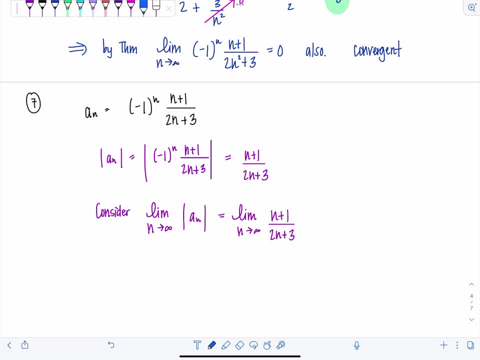 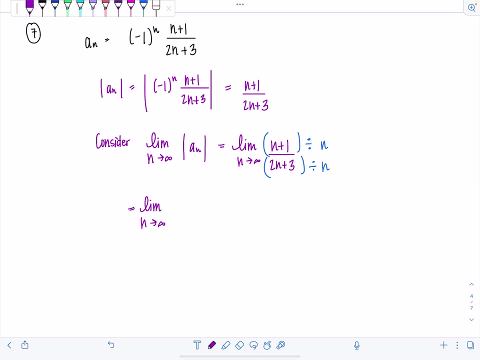 2n plus 3.. Same as before. I'm going to divide by the highest power of n from the denominator, But that's only n to the first this time. Oh, look how things are going to change. So now we have the limit, as n approaches infinity, of 1 plus 1 over n over 2 plus 3 over n. Let's 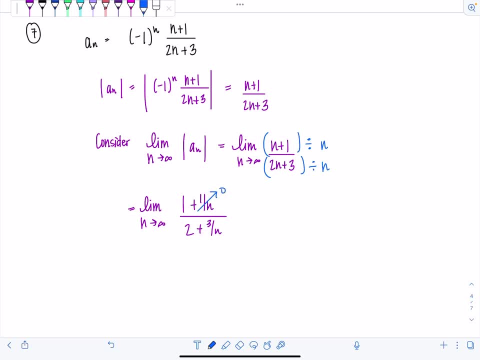 see, As n goes to infinity, 1 over n will approach 0.. 3 over n- where does that go? 0 also. So all I'm going to be left with is 1 over 2, and that makes me very sad, because that's. 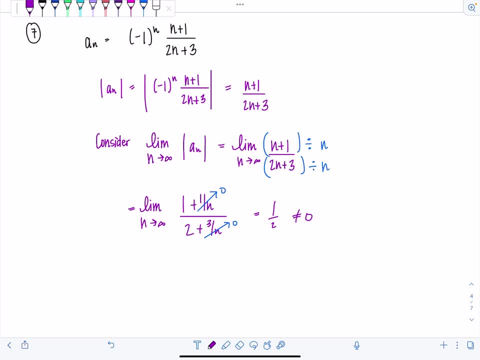 not 0.. So what can I say now? a? n actually is a divergent sequence, but we haven't justified that fully. Look at what's happening here. It's oscillating, yes. So if you consider the even terms versus the odd terms, you'll see precisely what's happening. okay, Even. 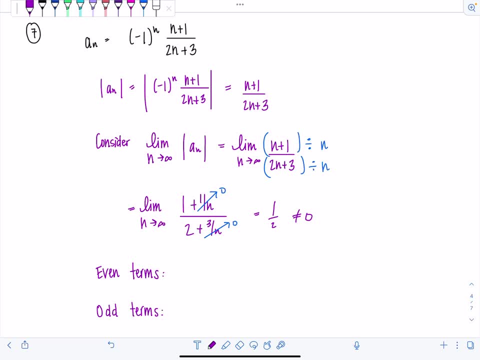 terms are all of the. You probably have a number of those like the second term, the fourth term, the sixth term, etc. So the even terms are defined by a sub 2n. They would be negative 1 to the 2n. I'm. 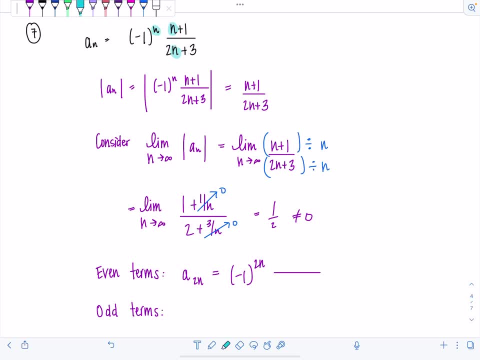 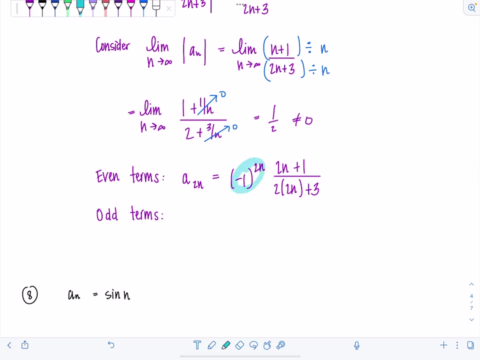 just substituting now 2n for n here. yeah, Okay, good, And then we would have 2n plus 1 over 2 times 2n plus 3.. Well, what results? Well, 1 to the 2n is just going to be positive. 1 because you're always raising it to an even power. So 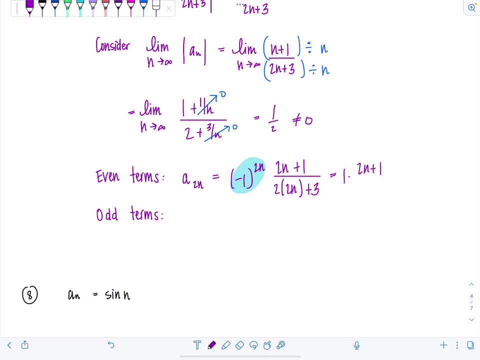 you're just going to have 1 times 2n plus 1 over 4n plus 3.. And it's not hard to show- let me just get this out of the way- it's not hard to show that the limit as n approaches infinity of a sub. 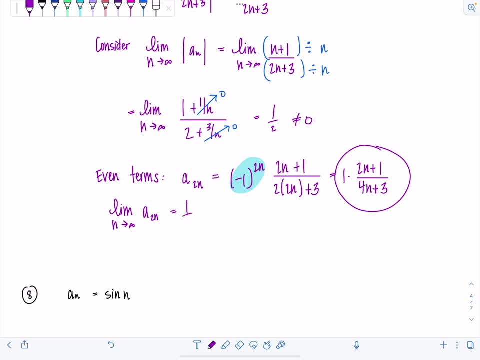 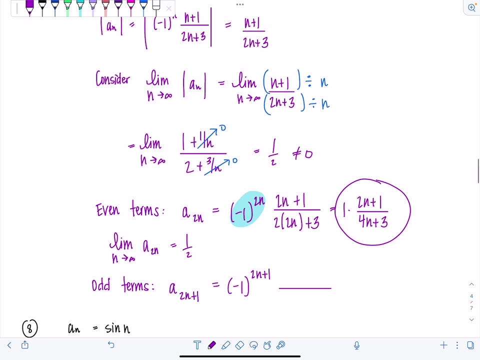 2n of these even terms is going to be positive 1. half The odd terms are going to be defined by a sub 2n plus 1.. So that would be negative 1 to the 2n plus 1.. Now this is going to get a little spicy. 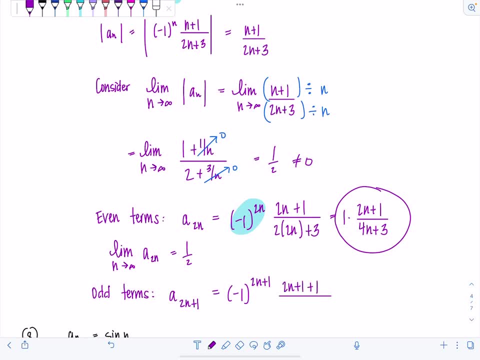 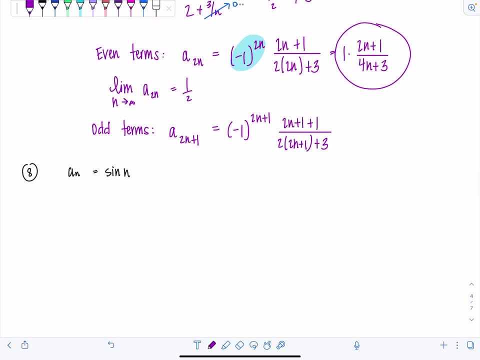 in the numerator, but you can handle it. It would be 2n plus 1 plus 1 over 2 times 2n plus 1 plus 3.. Well, what does that tell us? Move, I need some room. Negative 1 to the 2n plus 1 is always going to be negative 1 because you're. 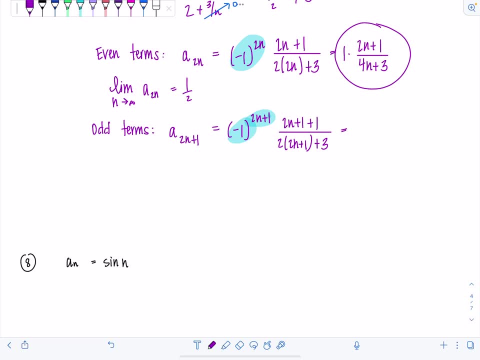 raising it to an odd power. So then you would have negative 2n plus 2 in the numerator over. this would be 4n plus 5.. And it's not difficult to show that the limit, as n approaches infinity, of the odd terms is equal to. 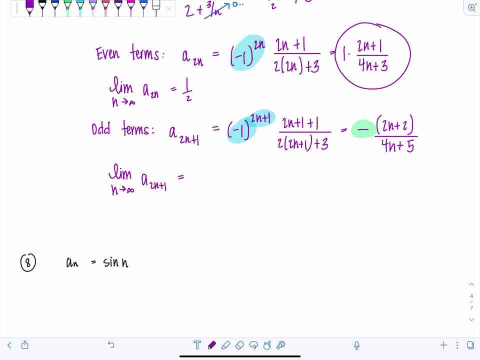 2.. See now how this negative stayed A negative 1 half. So basically there's another theorem when you study more advanced calculus that every subsequence in a convergent sequence must converge to the same limit. So since we have the even terms approaching positive 1 half and the 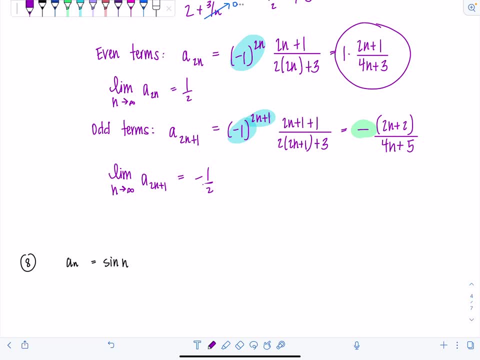 odd terms approaching negative 1 half. they're oscillating. Yes, it's bouncing around, So just imagine it's like this: Here's positive 1 half, Here's negative 1 half. Okay, And in the beginning the terms are big. 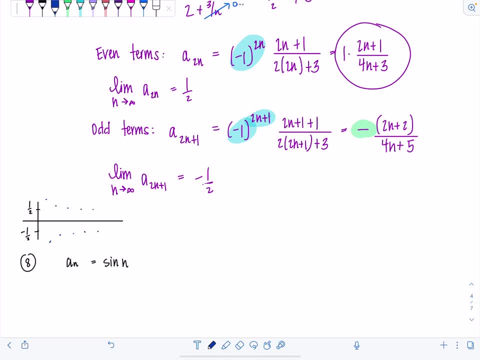 And then they shrink, but then they just keep bouncing like this, Bouncing, bouncing, bouncing, bouncing. So the limit doesn't exist. It's a divergent sequence. The theorem is specifically tied to 0 because only positive and negative 0 are the same value. 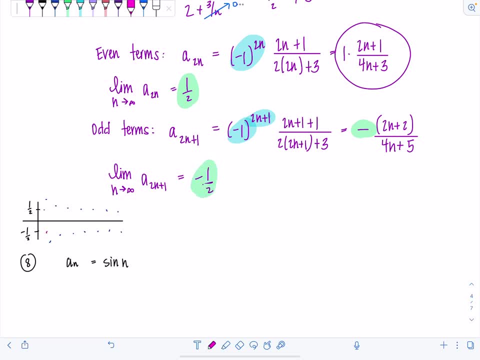 So that's why, when you take the absolute value, if the terms shrink, shrink, shrink and they're still bouncing, but they're getting close to 0, then we're good, right. The problem is when they approach a number other than 0, odd terms go one place, even terms go one place. So now that you've shown, 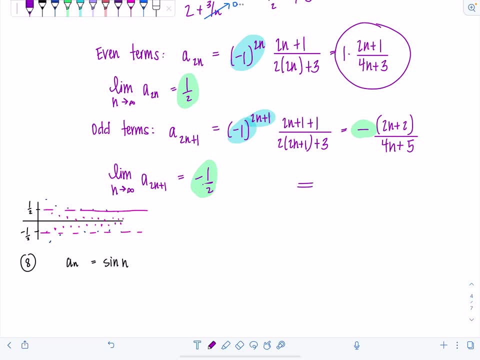 that the even and odd terms have different limits. then you can say: this means the limit as n approaches infinity of a n does not exist. Actually it oscillates, So it's divergent. That would be a full credit answer. in my class- I don't know how picky your professors are, So check. 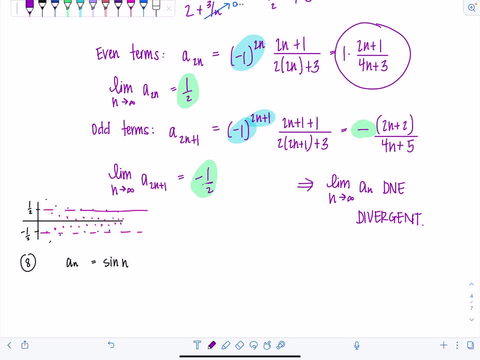 with them. Okay, Fabulous. Next one sequence: a: n is equal to sine of n. I mean, there's not a whole lot to say. Do we remember what the graph of sine looks like? I hope so. It's oscillating. 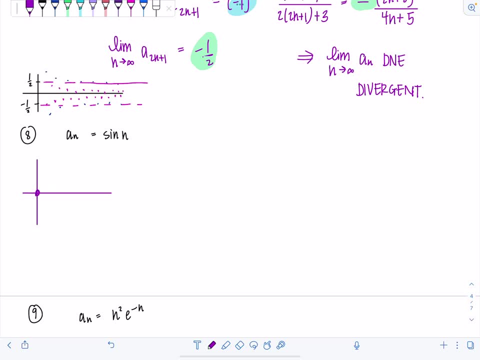 Now, I know this is a sequence, not a function, but sine of 0 would be here Sine of 1.. Sine of 1. It's less than pi. Sine of 2. Well, anyways, it's going to follow this shape, It's. 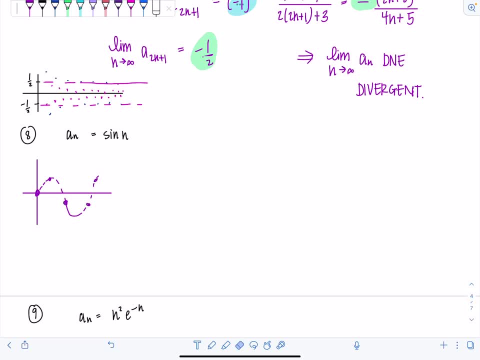 just going to be distinct points, And so it's oscillating And we can just say that the limit doesn't exist. How much work do you have to show? If you were in my class, you can just write the limit as n approaches infinity of sine n. It does not exist, It oscillates. If you want to write, 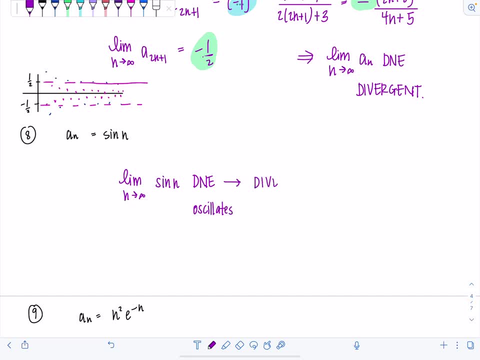 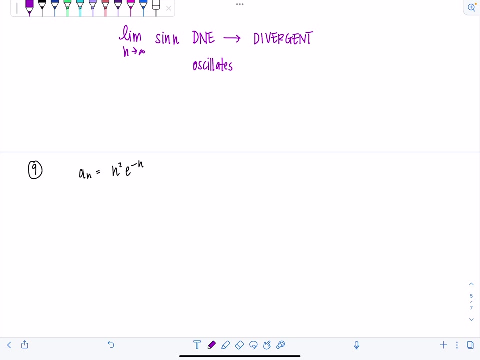 that down. Therefore, this sequence is divergent. It's bouncing around. It's bouncing around like a maniac. Okay, Let's look at a couple more cases where we can employ some of the methods I listed in the beginning of the video. So here we have a. n equals n squared times e to the negative n. 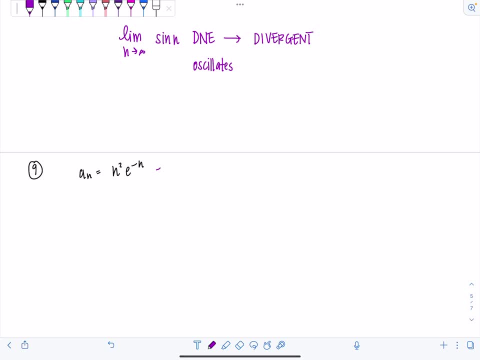 I always like to rewrite these negative exponents in the denominator, just because it helps me get an idea of what's going on better. So let's try to take the limit directly. Limit n approaches infinity. n squared over e to the n. It's not our typical rational expression where you just have 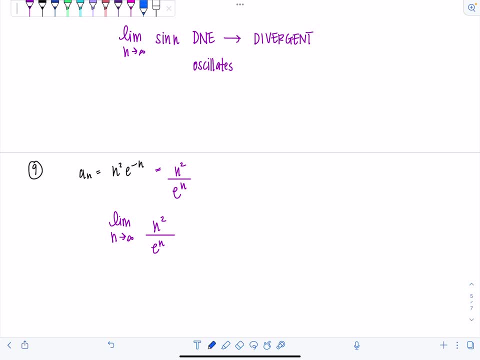 like polynomial in the top, polynomial in the bottom right. We've got that e to the n And as n approaches infinity, numerators approaching positive infinity, denominators also approaching positive infinity, So we actually have an indeterminate form. So let's look at a few more cases where we can apply L'Hopital's rule of the type infinity over. 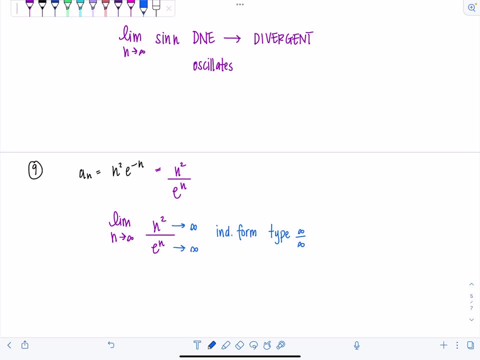 infinity. So it would be a beautiful moment to apply L'Hopital's rule, if only we were dealing with differentiable functions. and we're not. Sequences are definitely not differentiable. So what do you do? Well, you're a precise mathematician and you say: let f of x equal x squared. 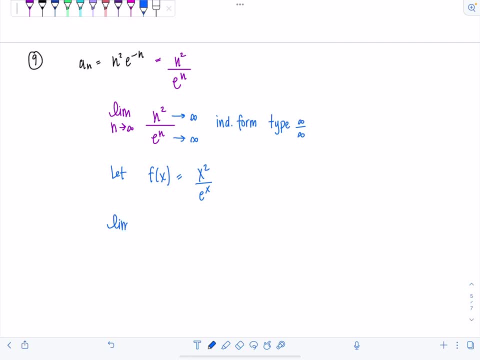 over e to the x. I'm just swapping out n's for x's, So now we're going to consider the limit as x approaches infinity of x squared over e to the x. I already have established that we have an indeterminate form of the type. 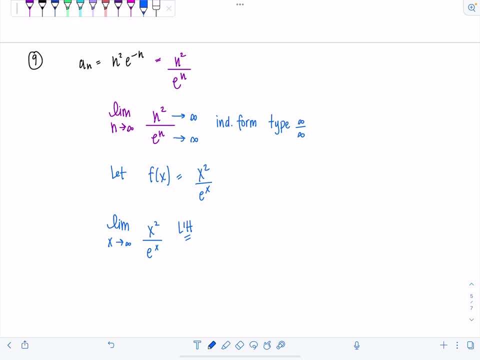 infinity over infinity. So I can apply L'Hopital's rule. And now we have the limit. as x approaches infinity Derivative of x squared is going to be 2x. Derivative of e to the x is still e to the x. 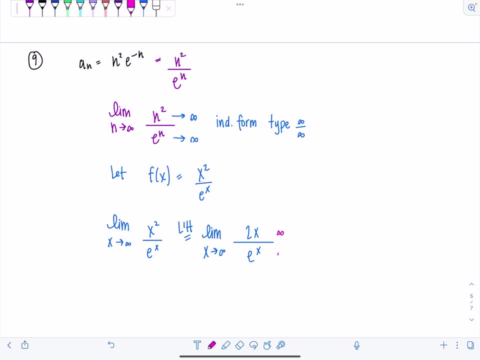 Well, I still have numerator approaching infinity, denominator approaching infinity, So let's apply L'Hopital's rule one more time. And now I have the limit, as x approaches infinity, of 2 over e to the x. Oh yay, So 2, that's just a constant. 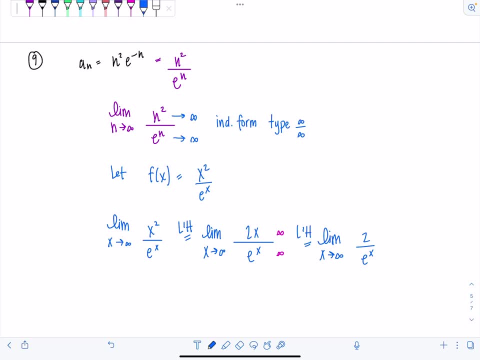 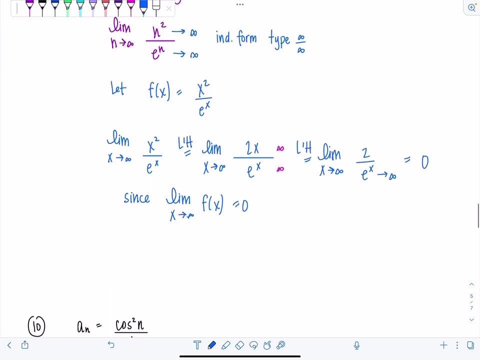 e to the x is approaching infinity, So constant over infinity, that is going to approach zero. So since the limit as x approaches infinity of f of x equals zero, then we can say that the limit as n approaches infinity of n squared e to the negative n equals. 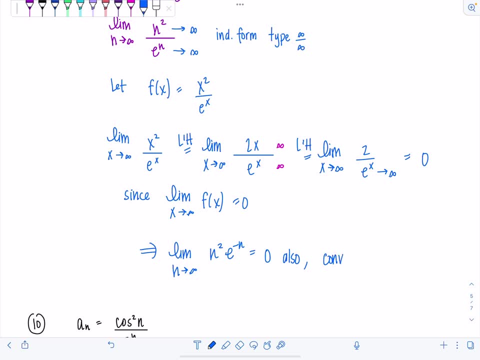 zero also. Therefore it's convergent And its limit L would be zero. All right, You have to be precise. I know it might feel silly, like All I'm doing is swapping out n's for x's. Well, too bad, okay. 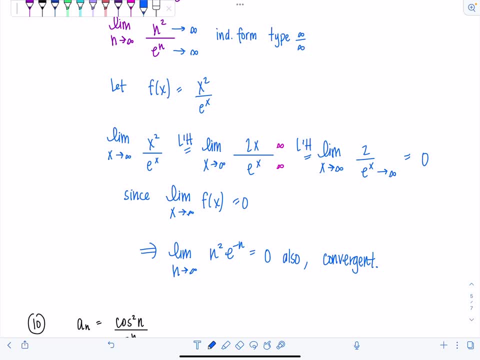 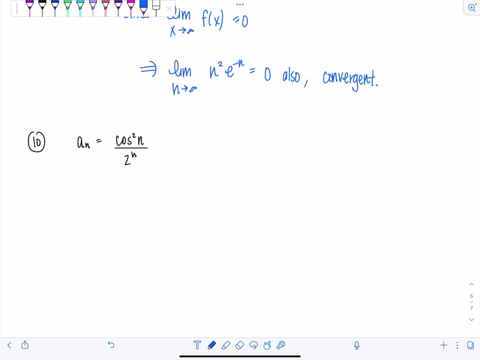 You're not allowed to use L'Hopital's rule unless you have a differentiable function. So just be glad we at least have L'Hopital's rule. It's just a couple seconds of your life, Okay, here's another. 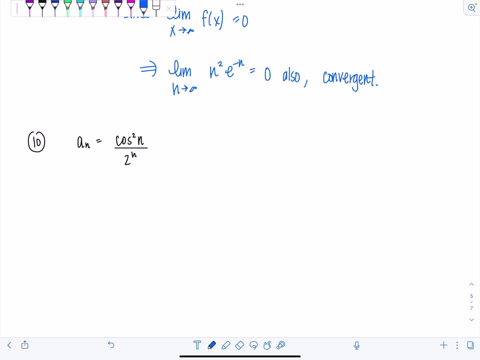 a n equals cosine squared n over two to the n. So if you try to take the limit directly, okay, cosine squared n? n. just think it's the same as cosine of n squared. And we know that cosine and sine, these oscillate. 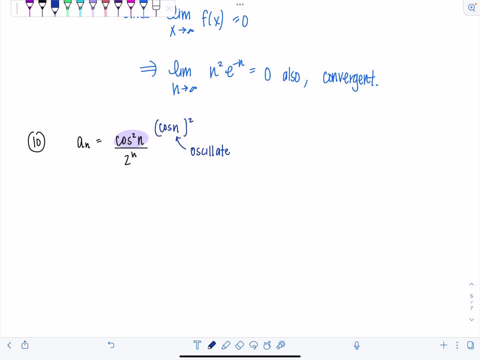 So the limit of the numerator doesn't exist. Two to the n, that's gonna approach infinity, And you might think, hmm, okay, so it's oscillating. I'm a little stuck there. I can't really use L'Hopital's rule. 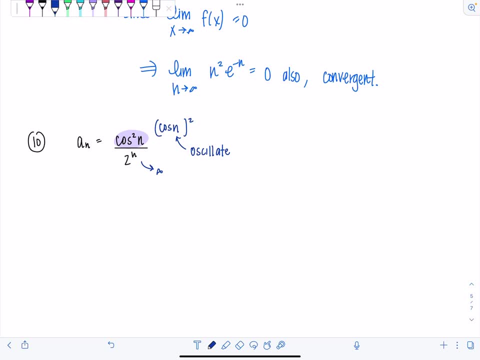 because if I keep differentiating cosine n, I'm just gonna keep getting back sines and cosines, sines and cosines. So it's not gonna help me. Maybe we should try the squeeze theorem, because cosine can be bounded right. 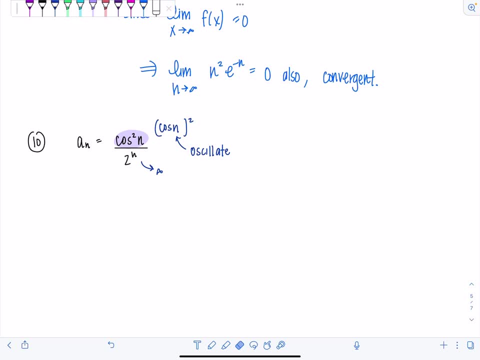 So it's actually cosine squared. Normally we say cosine of n is bounded between one and negative one, right? But if I square cosine it's never gonna be negative, right? Worst case scenario: the smallest it's gonna be is zero and it's still less than or equal. 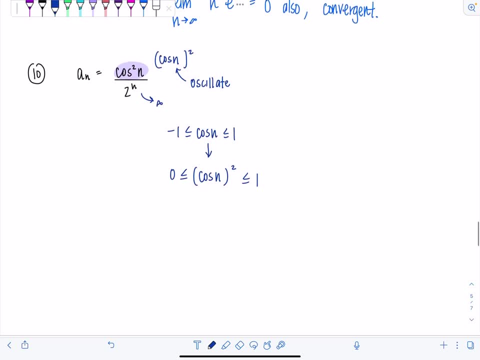 It's still less than or equal to one. And then I'm trying to make- I'm trying to squeeze the limit, So I'm trying to make the expression in the middle that's being squeezed match with this sequence. So I'm gonna divide everything by two to the n. 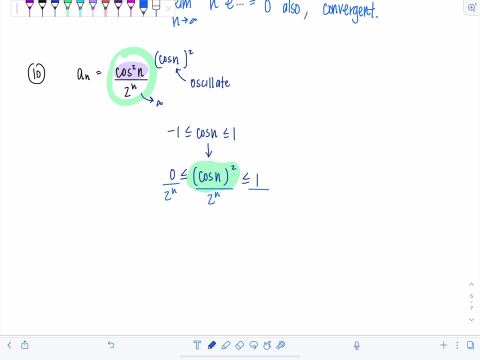 And two to the n is not negative, So I don't have to worry about the direction of the inequalities getting flipped or any of that right. Be careful: Since two to the n is greater than zero, the inequality is positive. It's preserved. 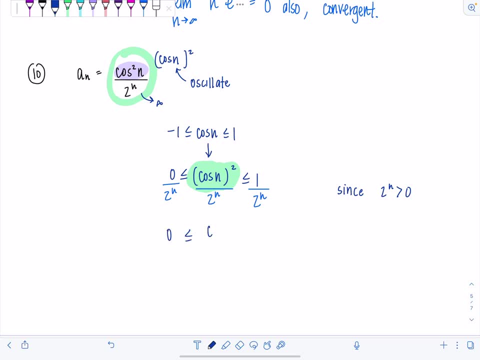 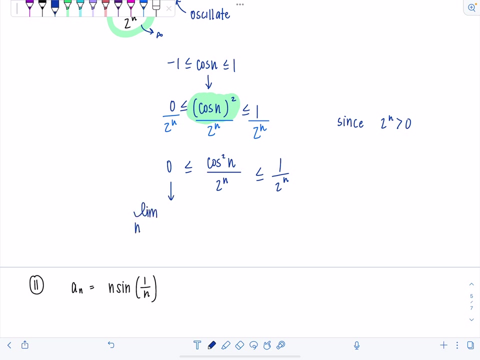 Zero divided by two to the n is still gonna be zero. This is- I'll write it to match the way it is in the problem. And then we have one over two to the n. So what does the squeeze theorem tell us? We'll take the limit of the lower bound. 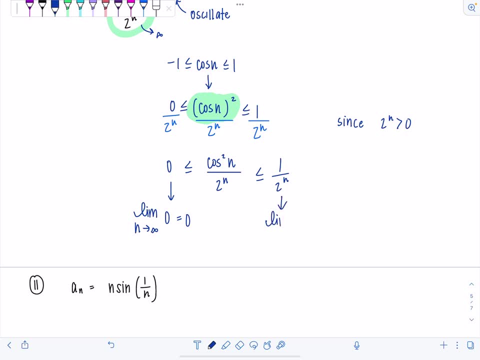 It's just a constant. Take the limit of the upper bound: one over two to the n. Well, two to the n is going to infinity right. One over two to the n is going to infinity right. One over something approaching infinity goes to zero. 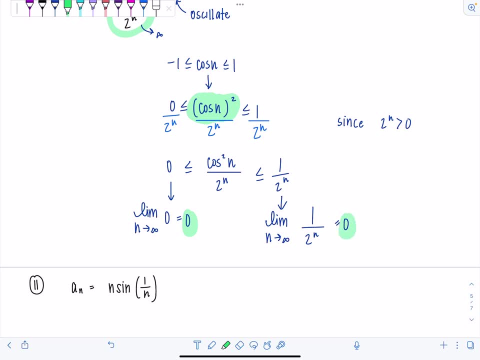 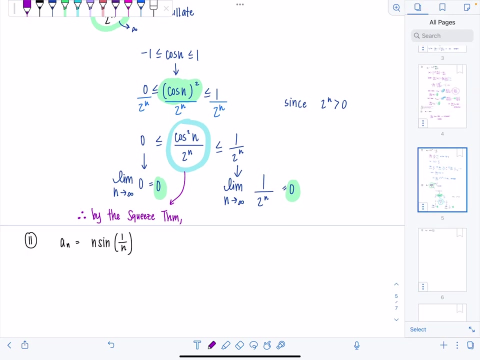 Notice, these are equal. So that tells us, by the squeeze theorem, fabulous things. Therefore, by the squeeze theorem, let me actually add a page. By the squeeze theorem, we're gonna have a square root of one over two to the n. 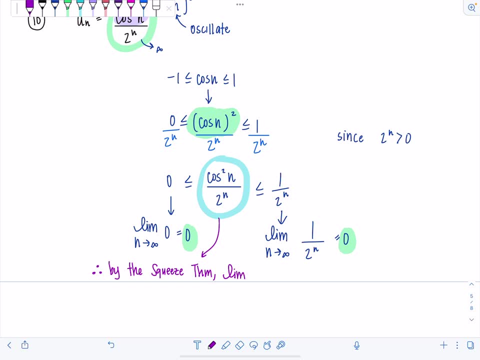 So we're gonna have a square root of one over two to the n. So we're gonna have a square root of one over two to the n. So we're gonna raise the theorem, The limit, as n approaches infinity of cosine, squared n over two to the n. 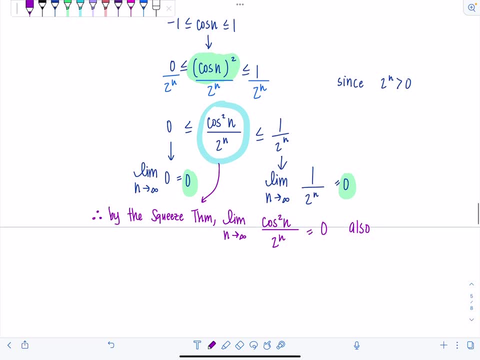 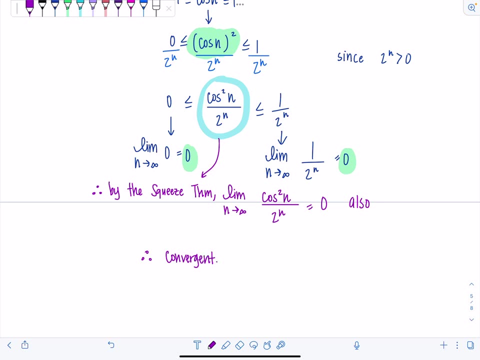 equals zero also and therefore it's a convergent sequence, And that I don't know if you can hear the little chiming music in the background. That was my wake up alarm. I woke up about two and a half hours before it. 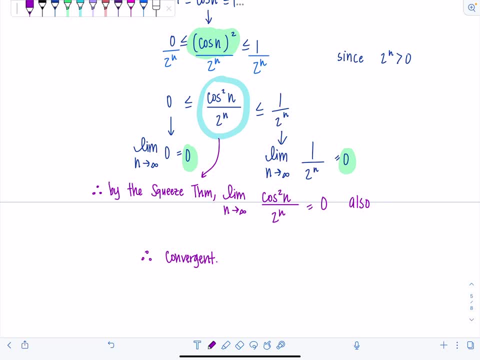 I was so excited to make this video for you all, So I'm actually gonna end it here, but we'll just do a part two with my alarm. more examples: okay, i'll turn off my alarm, get on with my morning or have to do a workout. 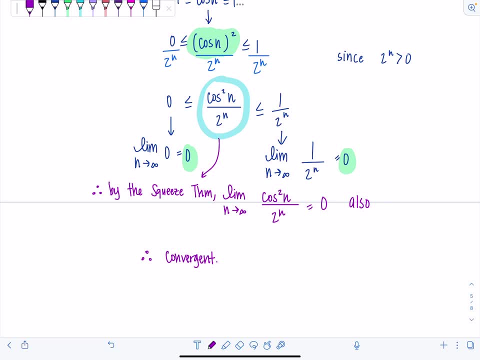 you know we do all the things over here. i hope you get some fitness in your life too. it's very good and give the video a thumbs up if you found it helpful. if you would like a part two, please comment down below if you feel like you're over sequences. you want something else? let me know too. 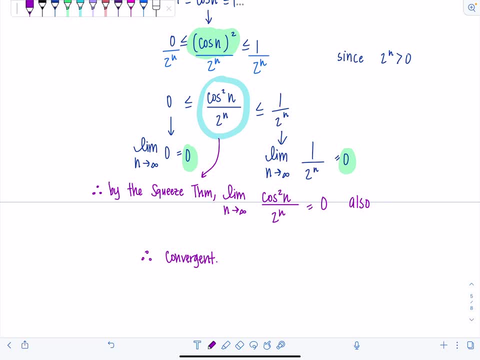 that's totally cool if you want access to exclusive content, quicker responses to your comments, etc. etc. if you're about the vip life, then click the join button. you can become a member to this channel also. you can catch me on instagram and tick tock at math tv. 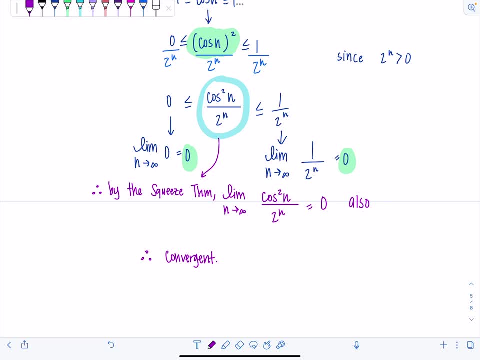 with professor v. i have all sorts of fun there, so stay tuned, you guys, subscribe and give this video a thumbs up if you haven't already. i'll see you all soon.